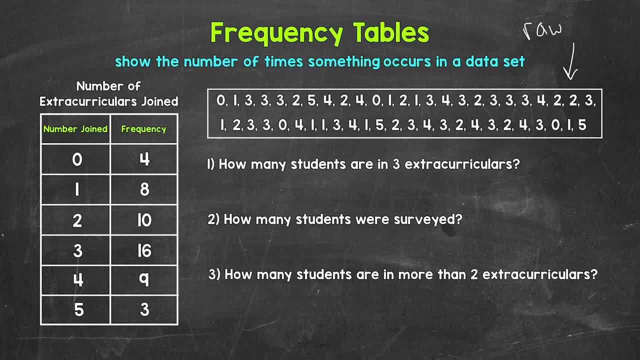 This is called raw data. As you can see, this is pretty difficult to interpret and understand, as is, And the frequency table will help us organize everything, and our table is right here to the left. Now the left column of the table. so this column right here represents the number of extracurriculars joined. 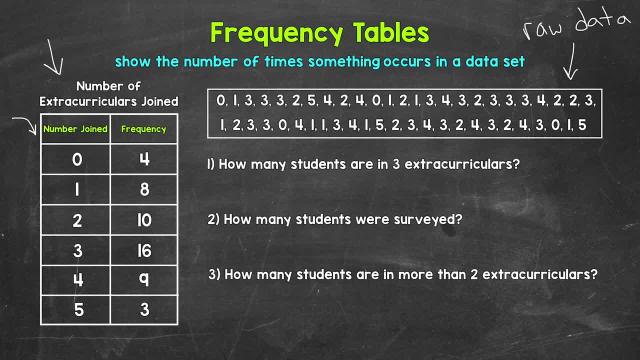 So 0,, 1,, 2,, 3,, 4 and 5.. As far as how I determined which numbers to put there, I just went from the smallest number in value in the dataset. So zero, one, two, three, four and five. 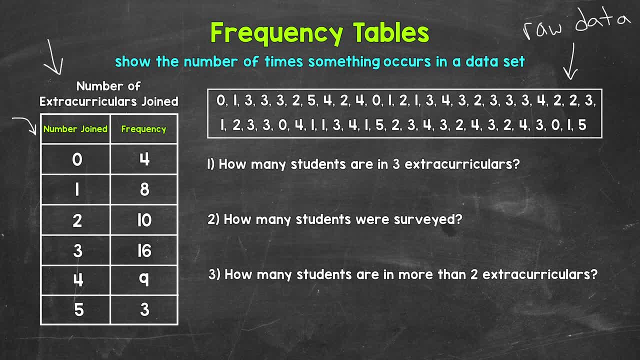 I set zero, one, two, three, four and five. I set zero, one, two, three, four and five zero to the greatest number in value, five. Now, this is considered ungrouped data because we have 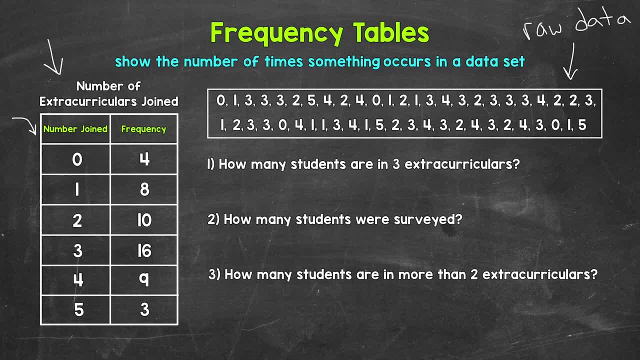 individual values in this column, not groups or ranges. You'll see what I mean by groups, grouped data, when we get to that example. You'll see the difference And then on the right side, the right column, right here, we have the frequency, the number of times those values. 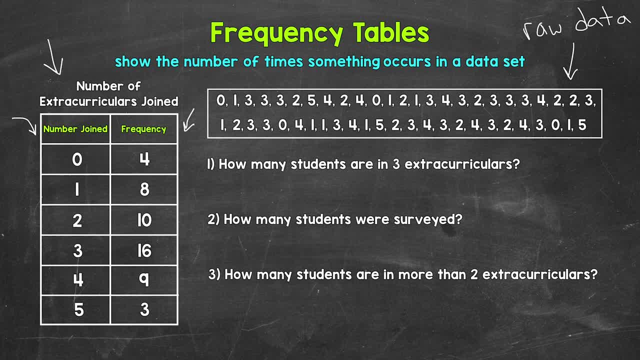 show up within the data. So, looking at the table, let's read this table here. How many students aren't in any extracurricular activities? So zero extracurriculars. We look right here: number joined zero, There are four students. So four students aren't in any extracurriculars. 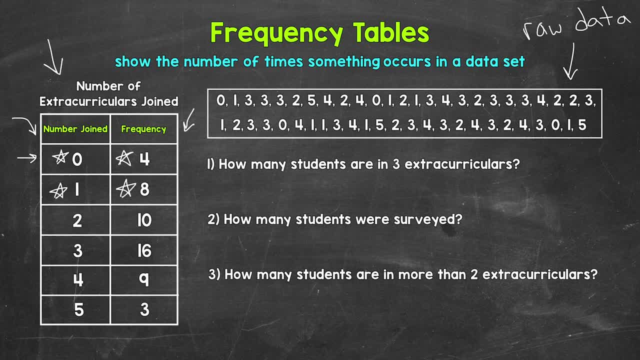 How about one? Well, there are eight students in one extracurricular activity. How about two? Well, 10 students. Three, there are 16 students. Four, there are nine students, And then five, there are three students. So you can see that this frequency table really helps organize and 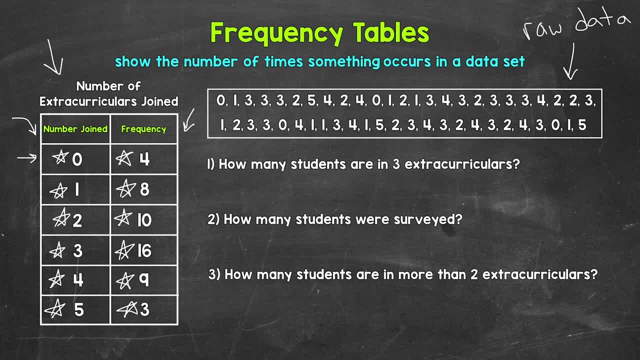 present the data in a meaningful and easier to understand way than to look at the raw data. Now let's answer some questions regarding the data, Starting with number one, where we have how many students are in three extracurriculars. Well,